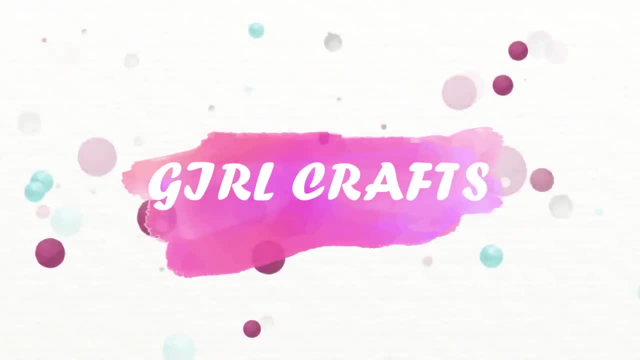 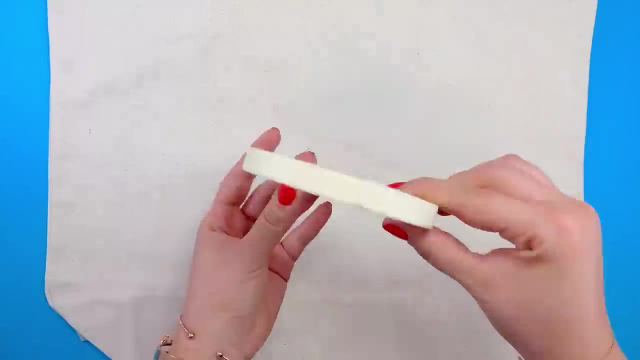 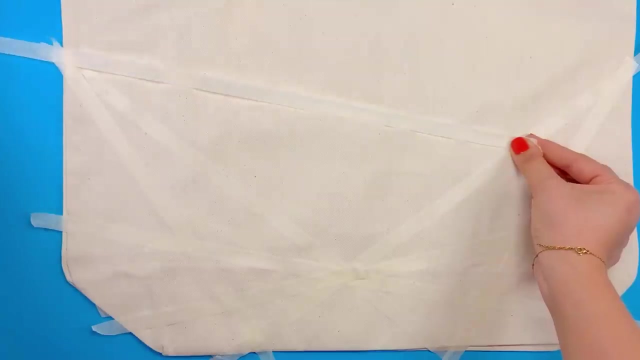 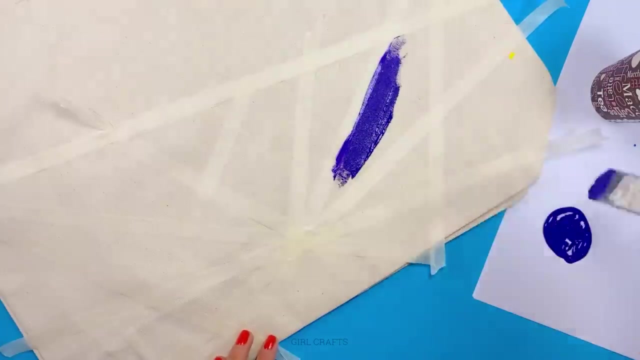 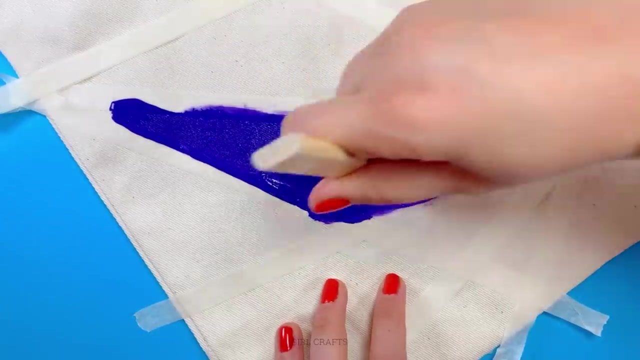 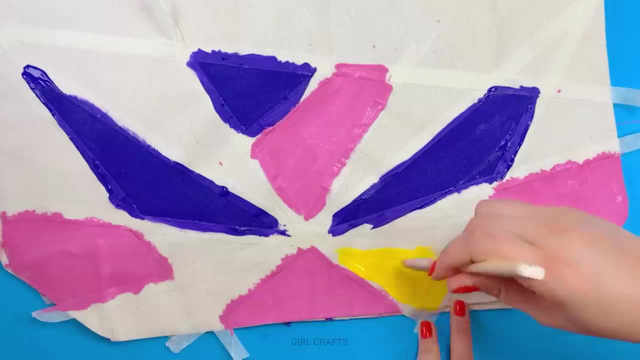 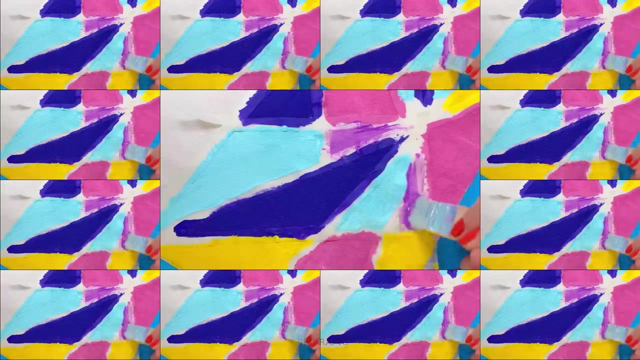 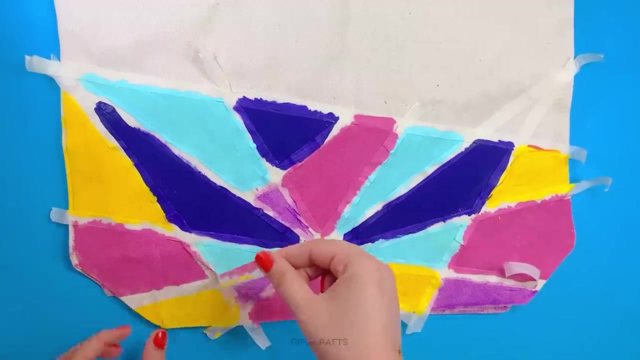 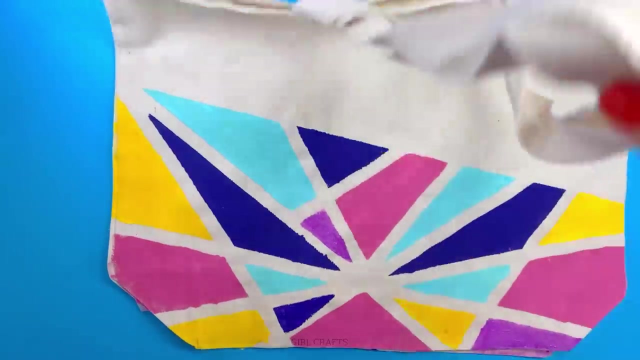 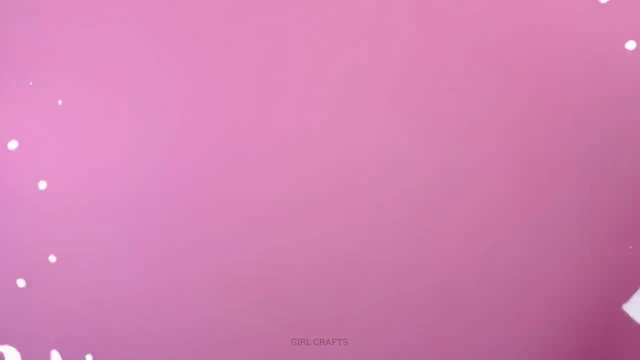 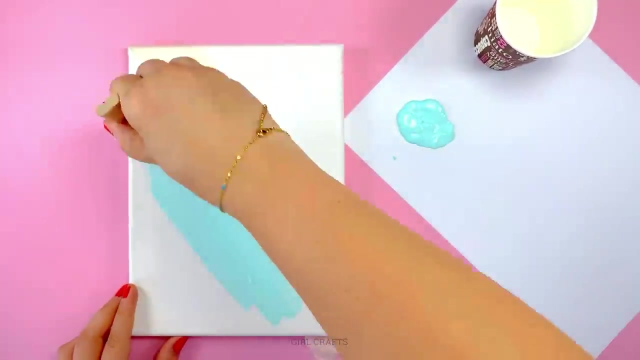 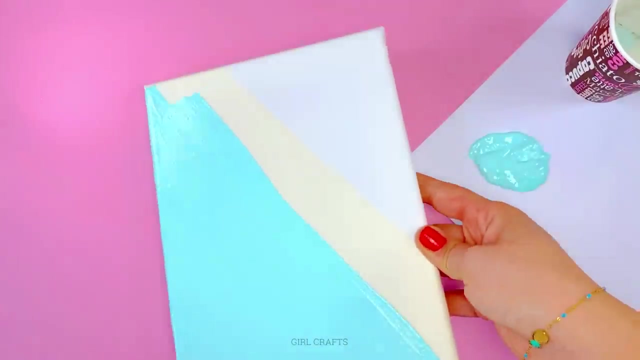 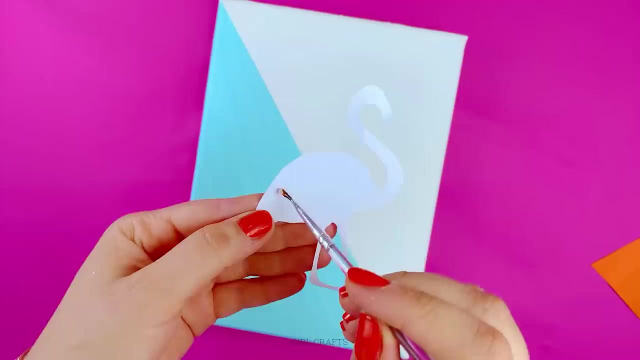 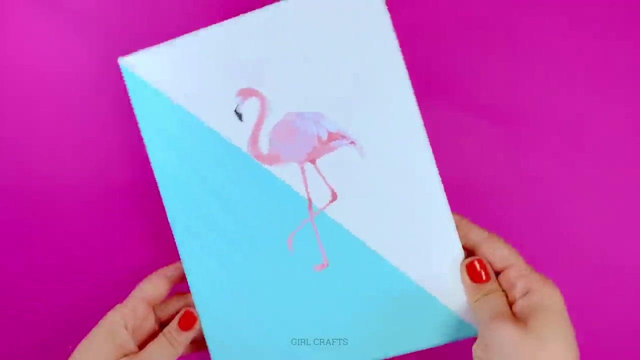 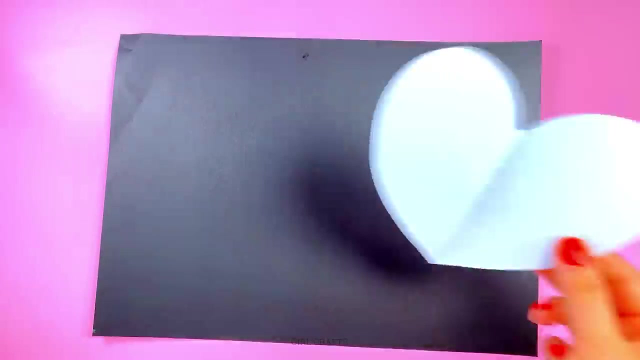 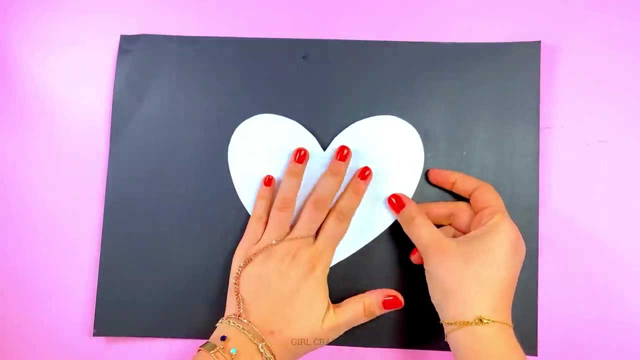 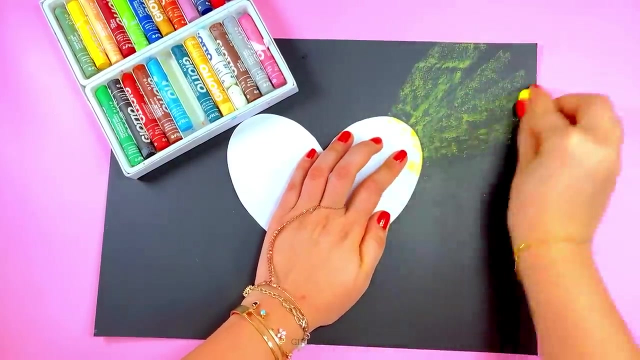 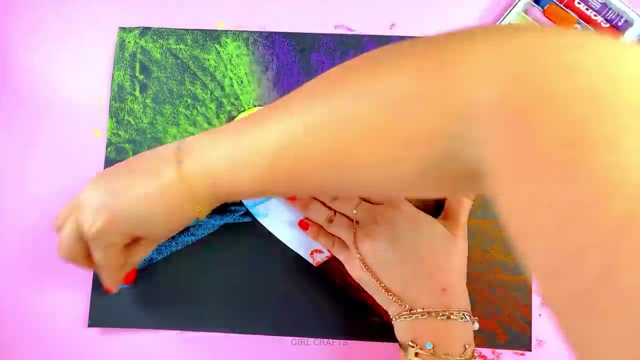 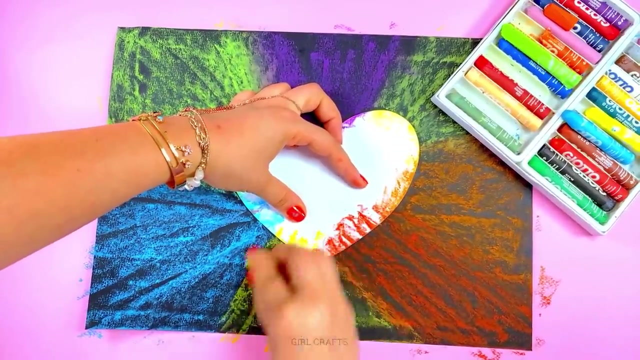 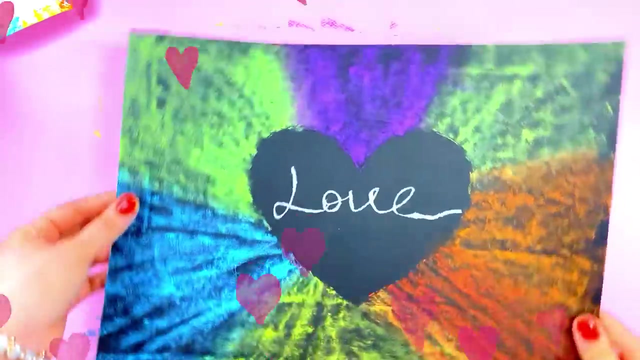 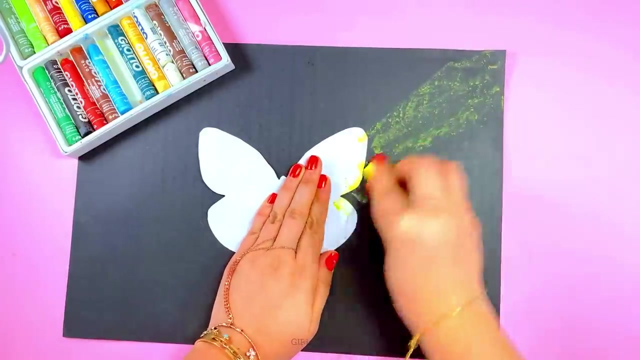 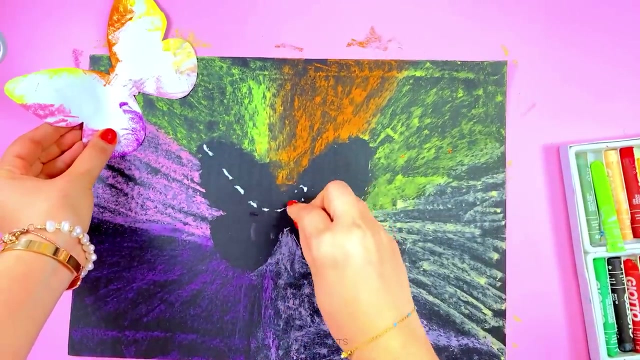 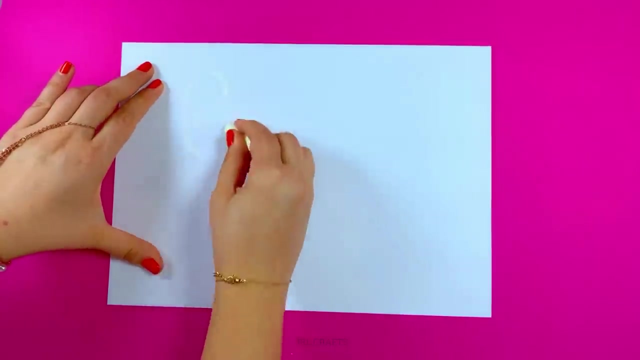 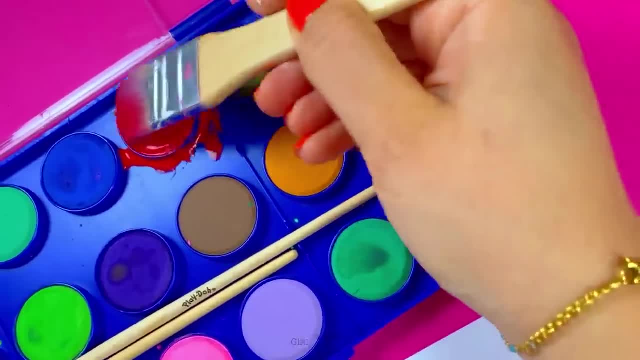 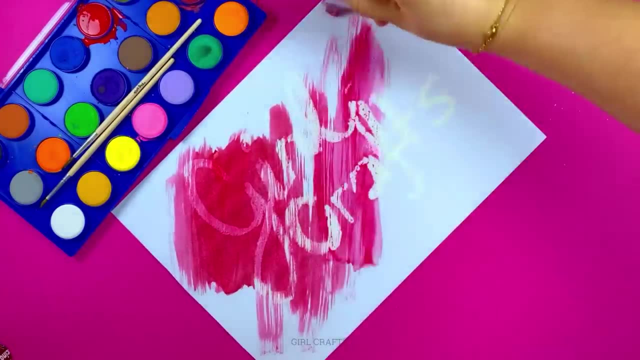 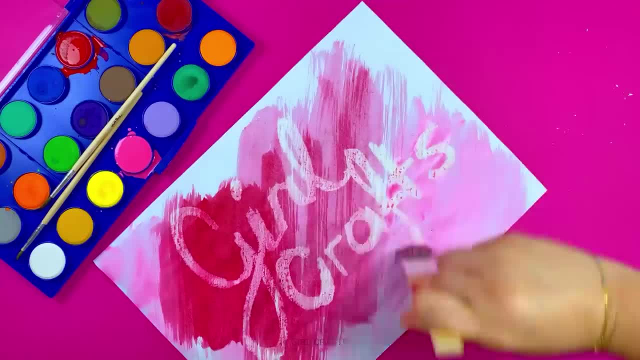 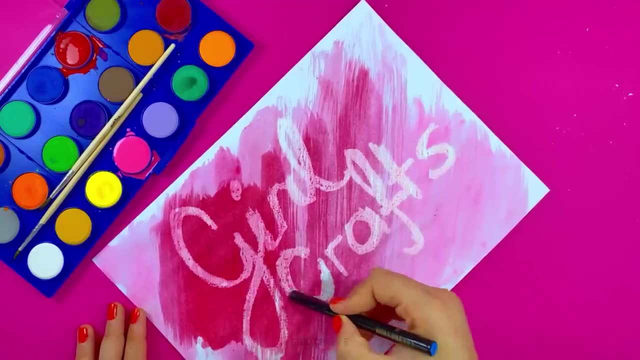 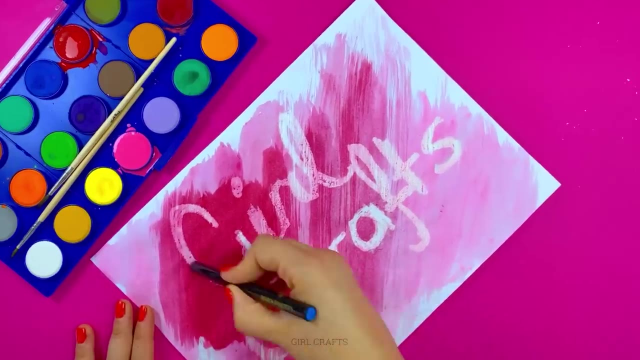 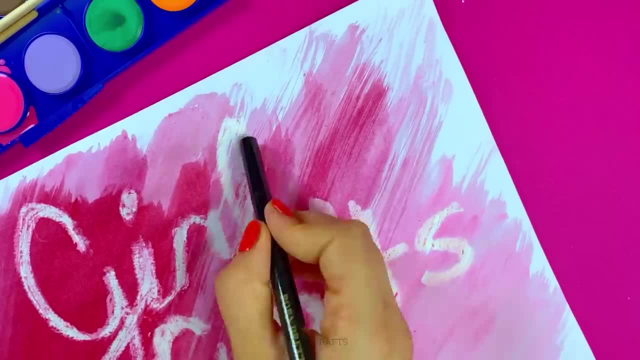 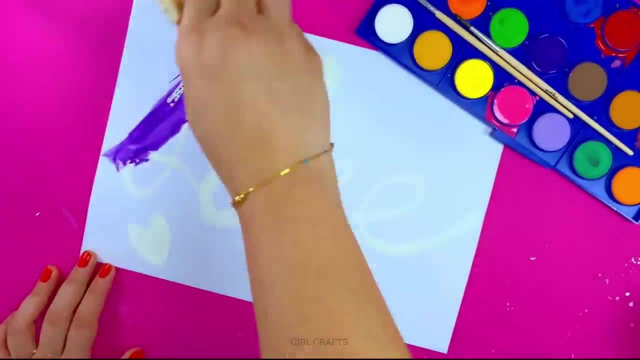 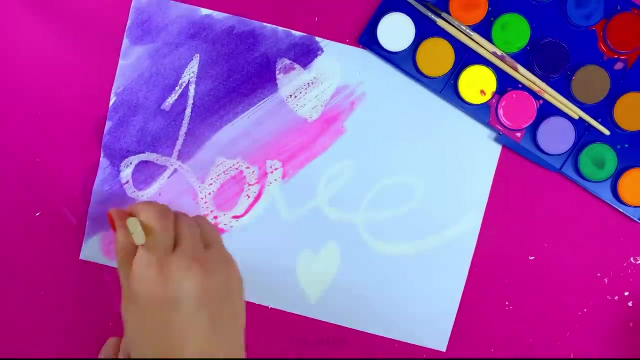 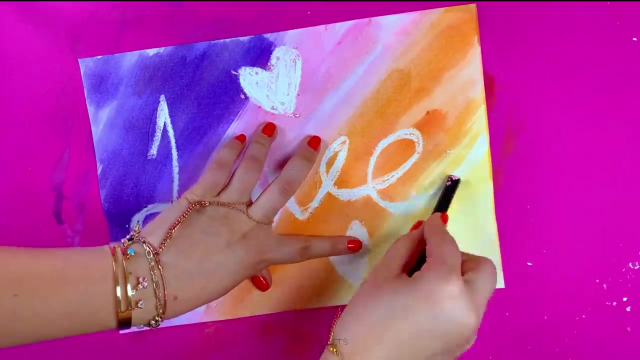 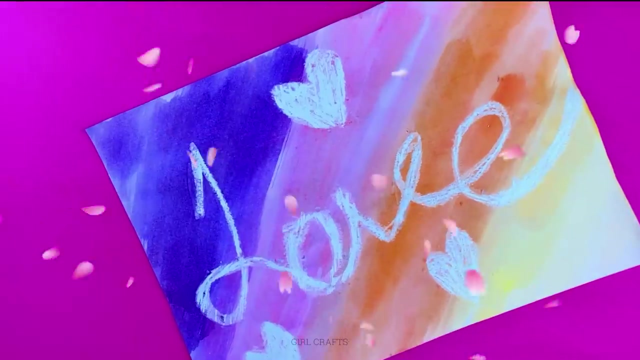 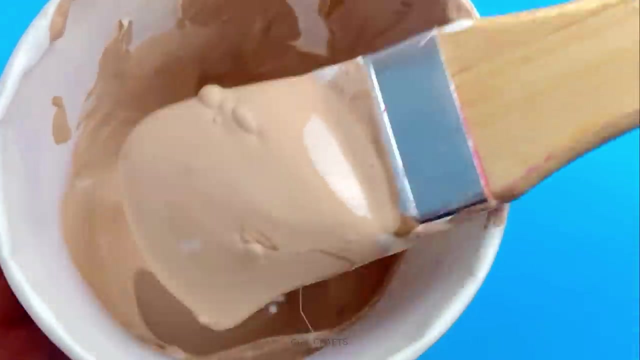 So glad we met On that day. You took my breath away. If I could harness time, Maybe I would hit rewind Or maybe pause, Cause I'd like to stay a while. A face like yours I won't forget. A face like yours, So glad we met On that day. 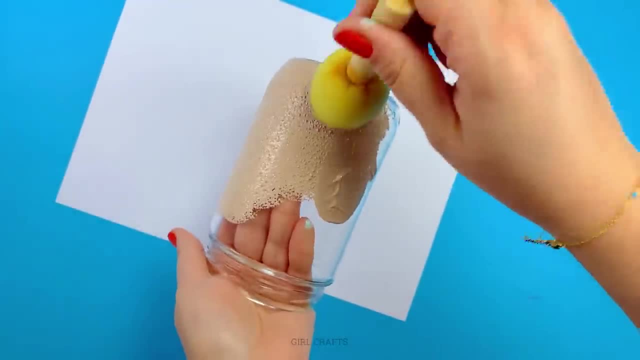 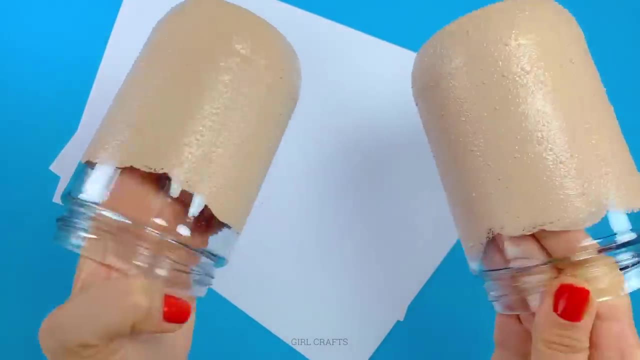 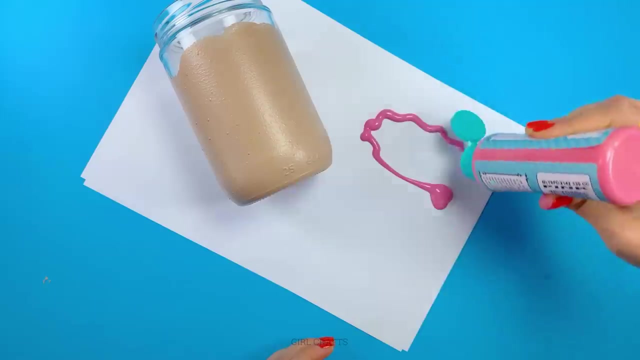 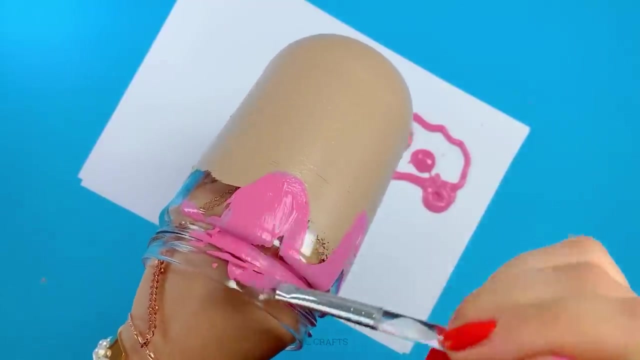 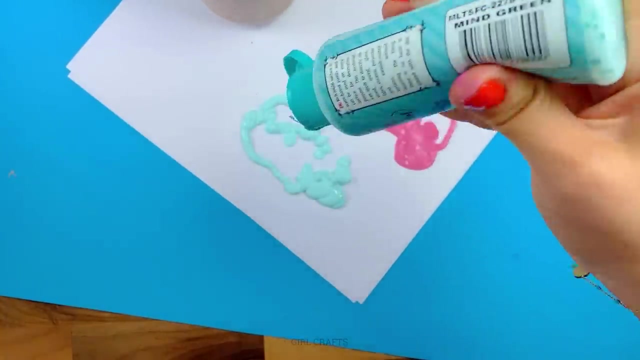 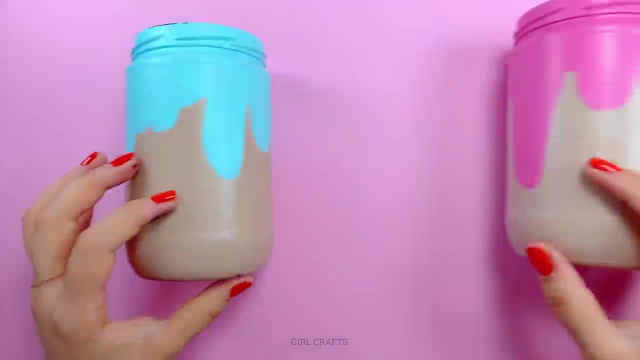 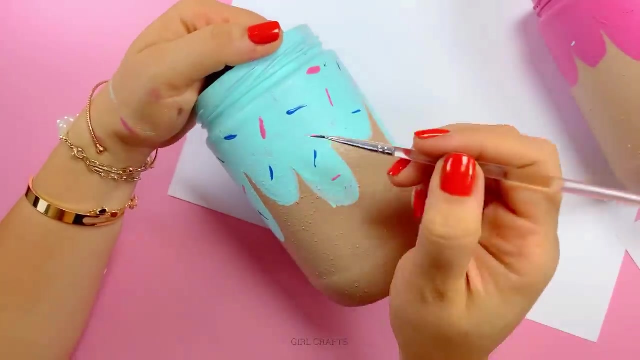 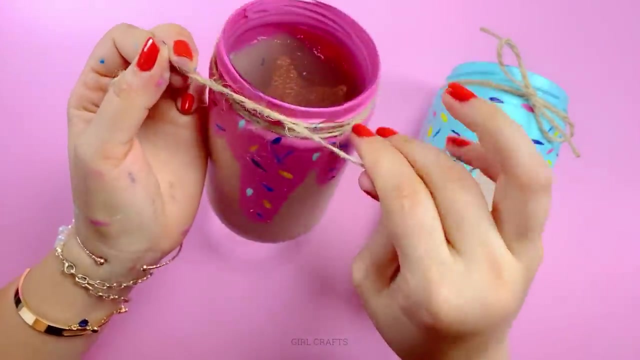 You took my breath away. A face like yours. A face like yours, I won't forget. A face like yours. So glad we met On that day. You took my breath away. A face like yours. I won't forget. A face like yours. So glad we met On that day. 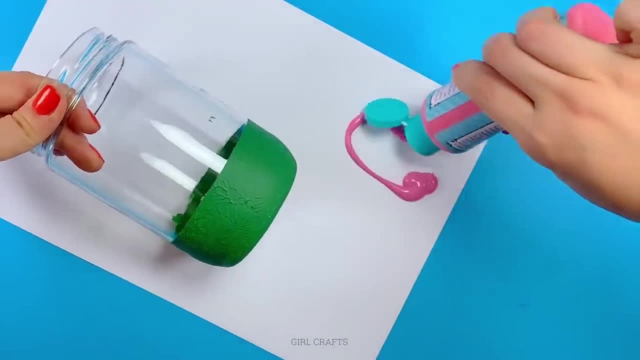 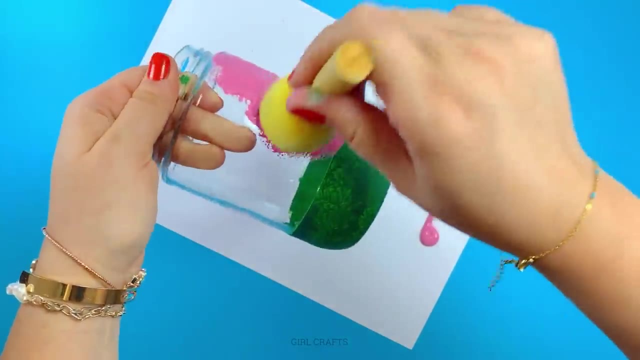 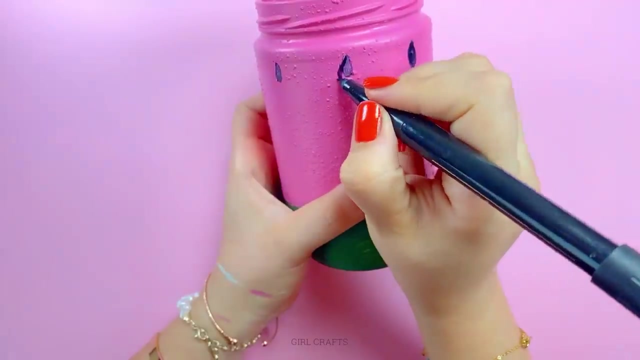 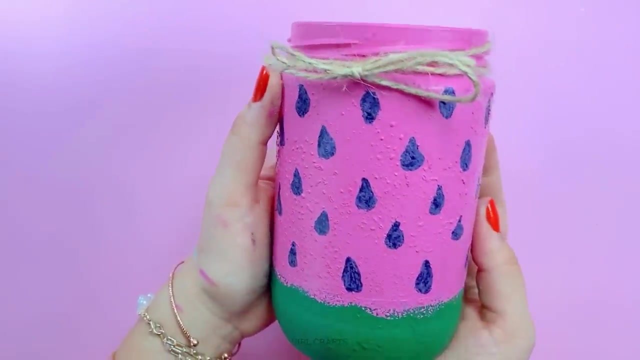 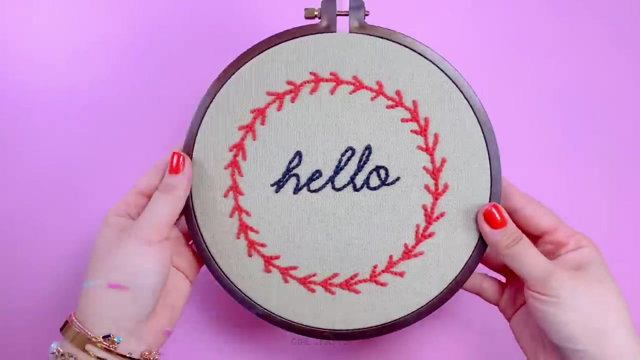 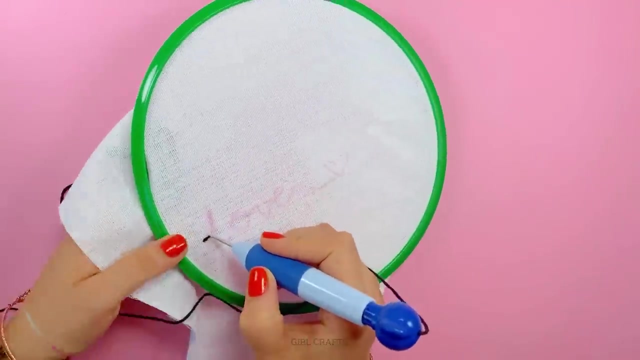 You took my breath away, A face like yours. I won't forget A face like yours. A face like yours, So glad we met On that day. You took my breath away. If I could harness time, Maybe I would hit rewind Or maybe pause, Cause I'd like to stay a while. 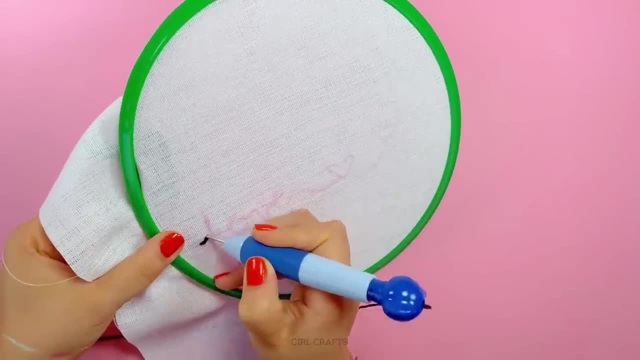 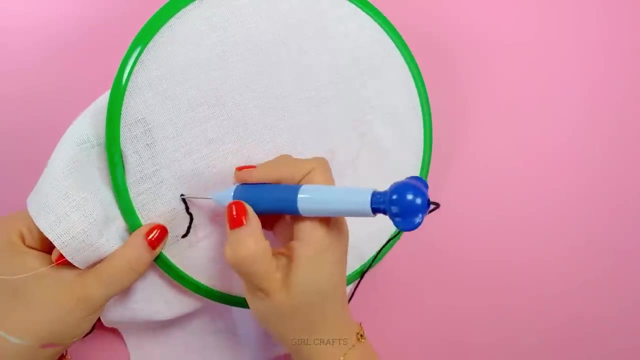 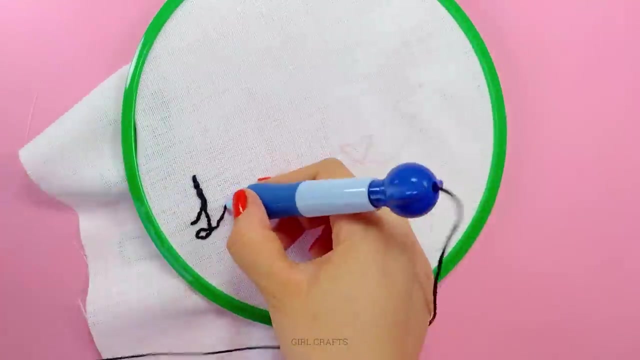 All day a while. Ooh-ooh-ooh, ooh-ooh-ooh, Ooh-ooh-ooh-ooh-ooh, Ooh-ooh-ooh, ooh-ooh-ooh, Ooh-ooh-ooh-ooh, Don't um, don't hesitate. 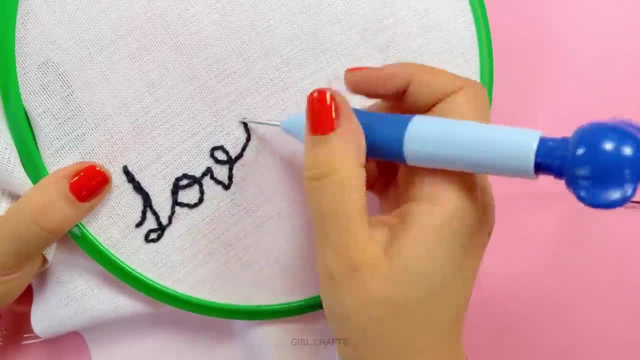 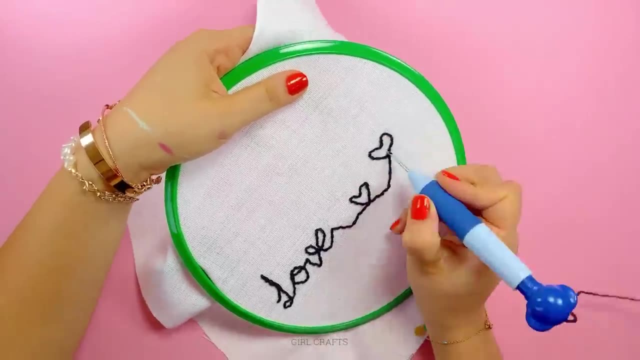 It's only harder the longer you wait. I know we only have so-and-so. It's only harder the longer you wait. I know we only have so-and-so. It's the rake now, while the iron is hot. Before it's gone, the moment lasts. 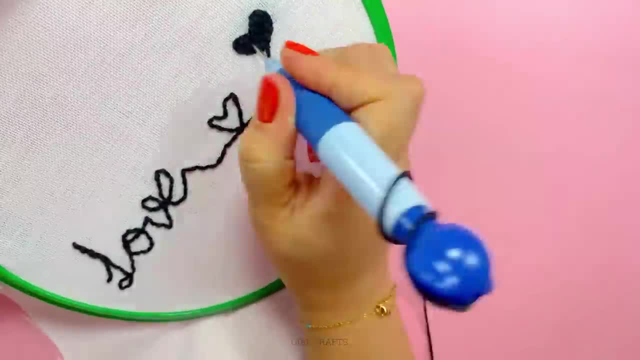 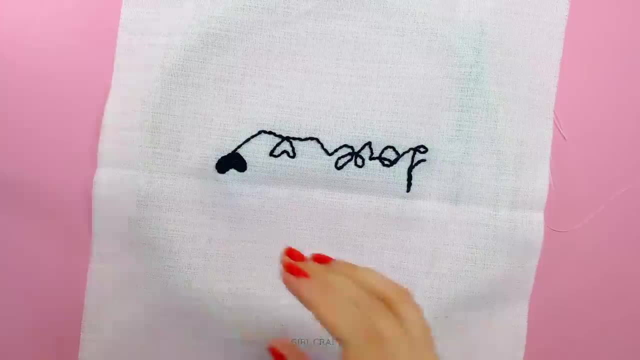 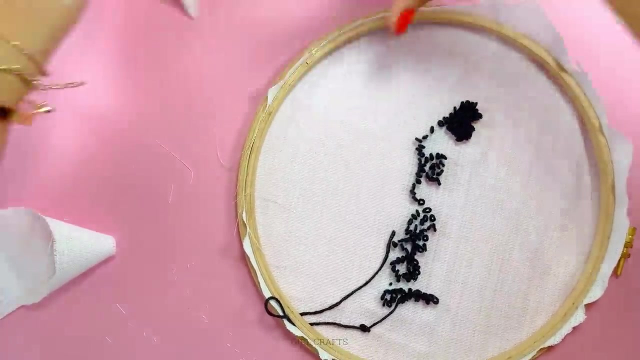 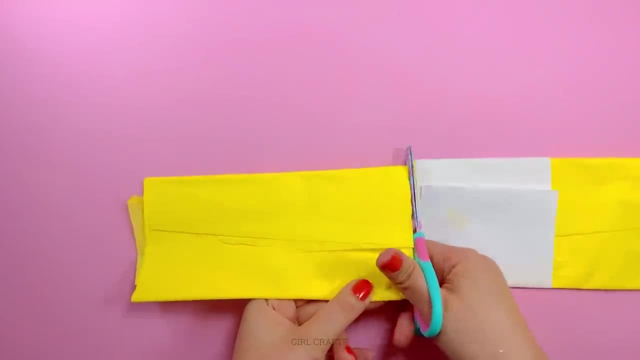 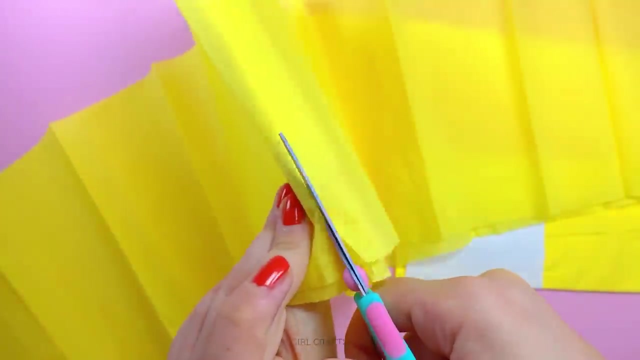 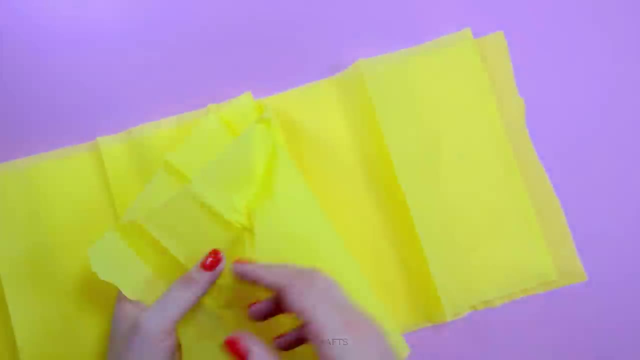 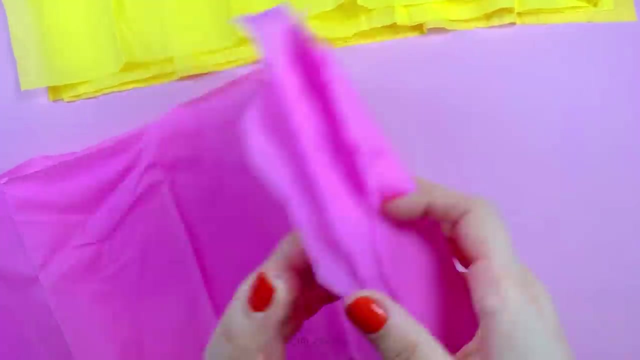 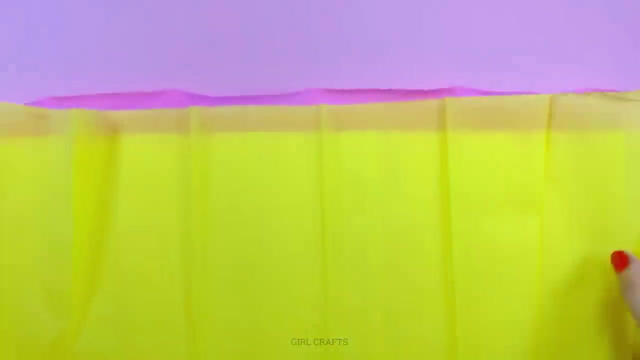